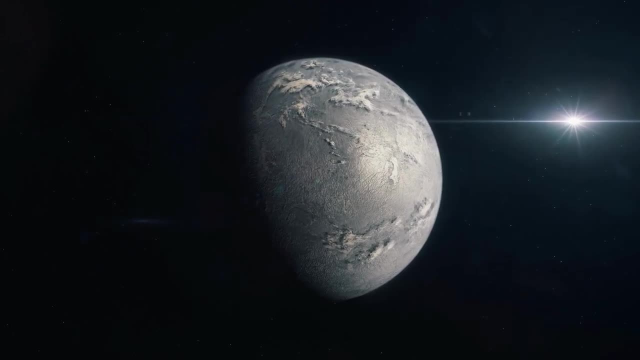 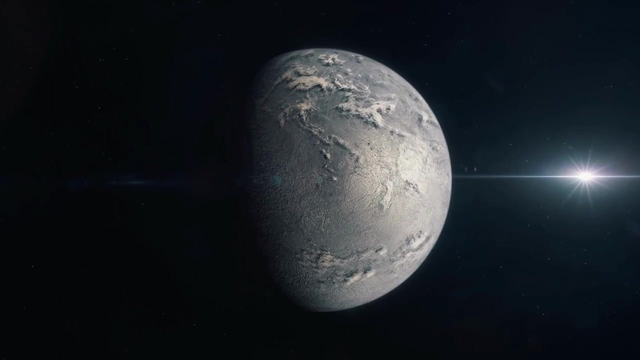 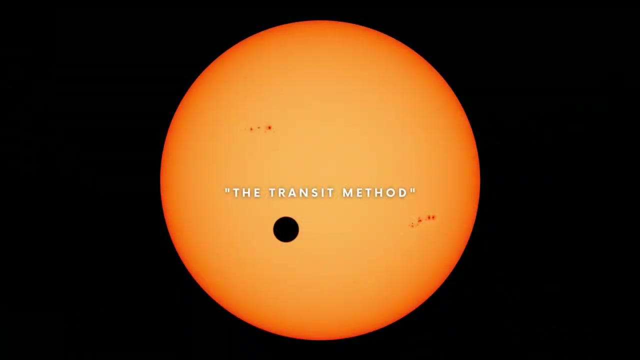 in recent years. by astronomers, Exoplanets are verified by a variety of techniques, the majority of which are indirect in nature. The following method has been used to find more than half of the exoplanets ever discovered: The transit method, While the radial velocity 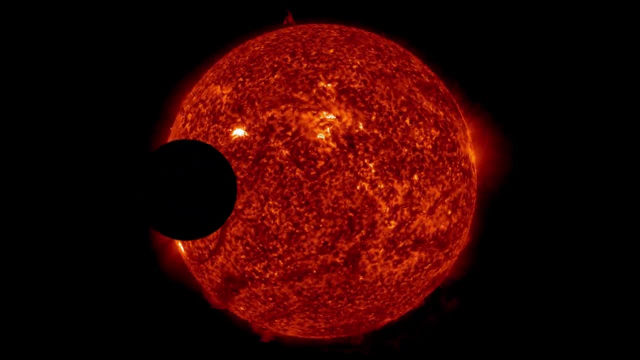 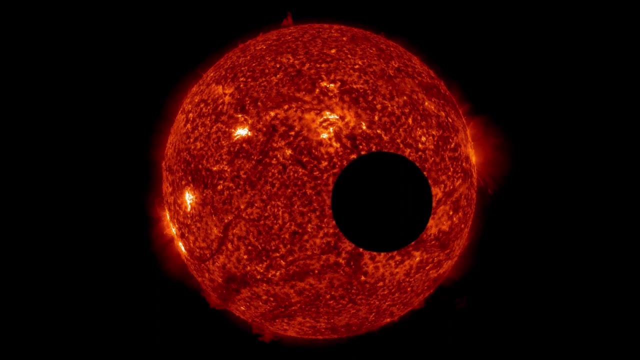 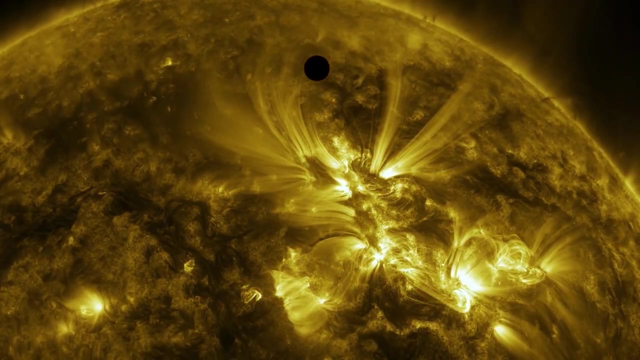 method can determine a planet's mass. the transit photometric method can determine its radius. The first transit photometry detections were made in 1999.. When a planet passes in front of its parent star's disk, the observed visual brightness of the star 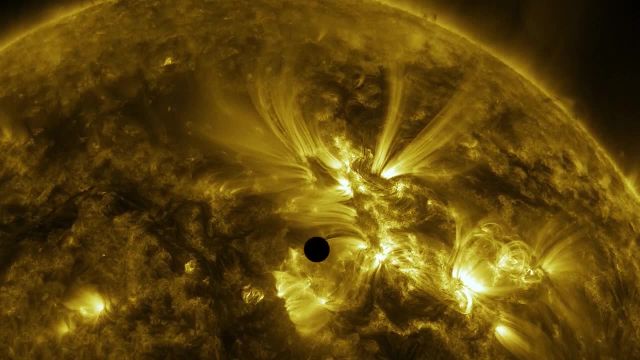 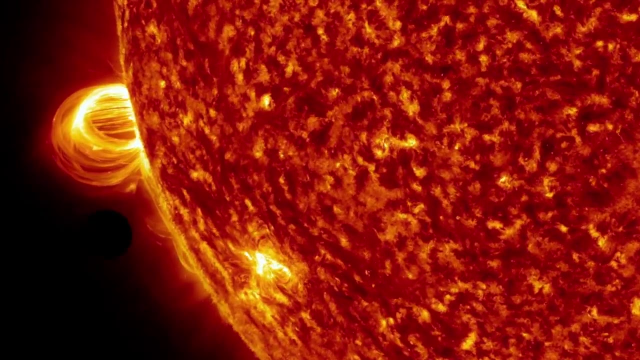 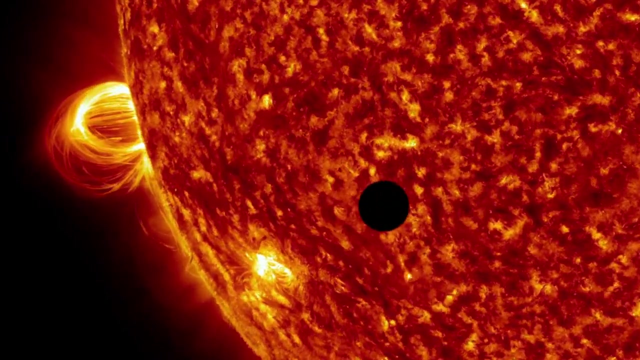 decreases slightly or dims, depending on the relative sizes of the star and the planet. The amount a star dims during a transit is proportional to the size of the star and the planet. A small planet passing through a large star causes only a slight dimming, whereas a large planet passing through a small star causes only a slight dimming. When a planet passes through a large star- a planet passes through a larger one than a large planet passes through a huge one- The elevation of the star goes up by the first beam remains equal to 1mm in diameter. 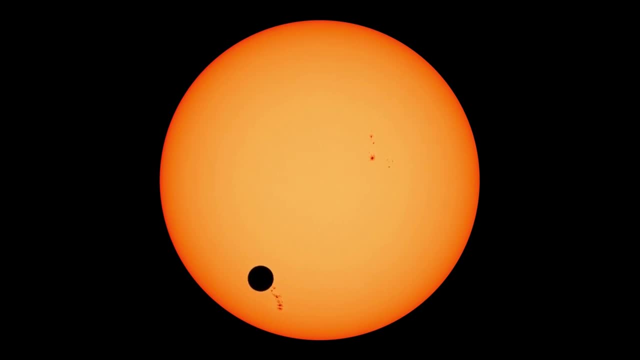 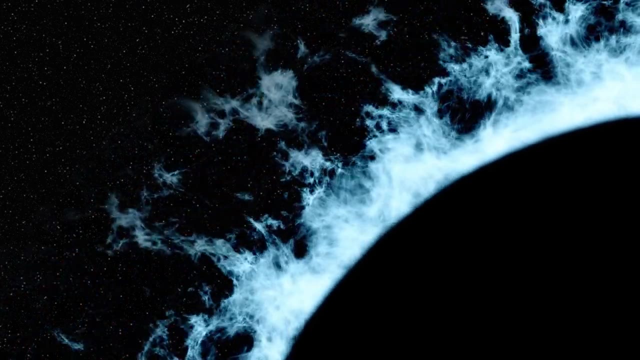 Transits can assess and determine a variety of exoplanet characteristics. The size of the exoplanet's orbit can be calculated by calculating the time period it takes to orbit once, and the size of the planet itself can be calculated by calculating how much. 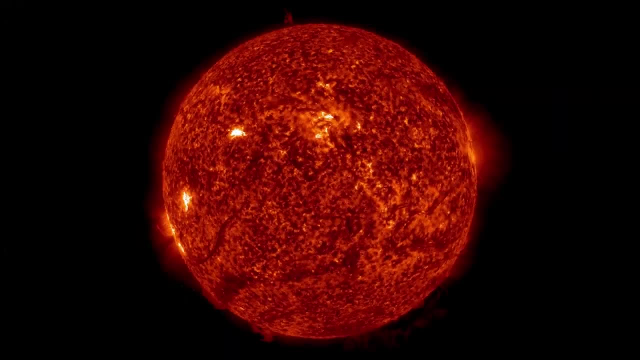 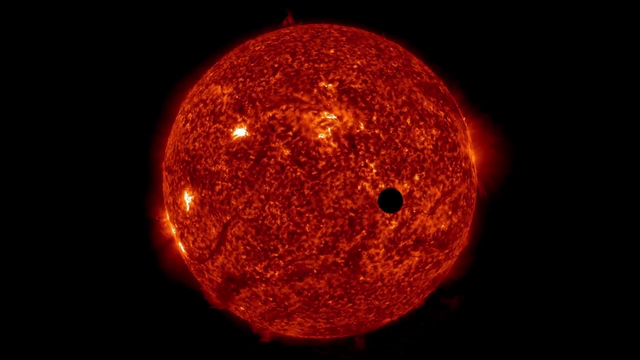 the star's brightness has been reduced. These changes in brightness are characterized by very small dips and for fixed periods of time. usually indicates, though, subtle changes may occur quickly. But even if the star's brightness goes, bamboo춘, neighborhood of 1- ten-thousandth of the star's overall brightness, lasting only a. 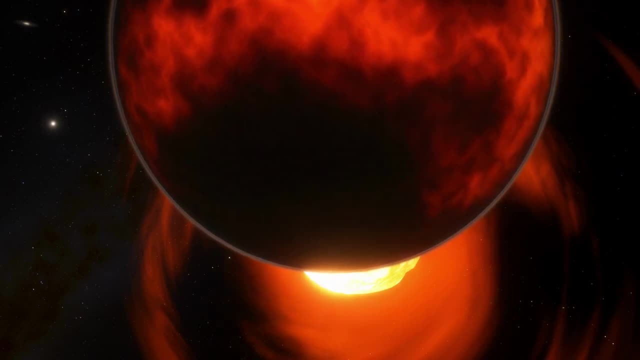 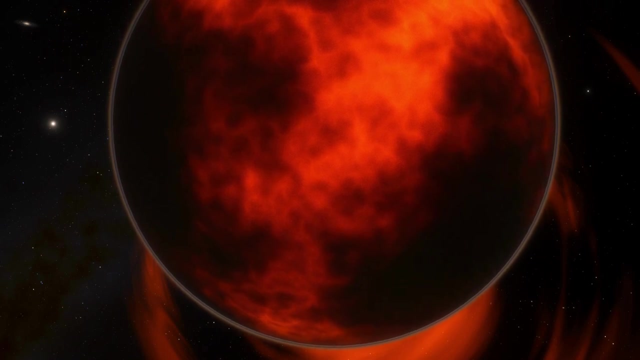 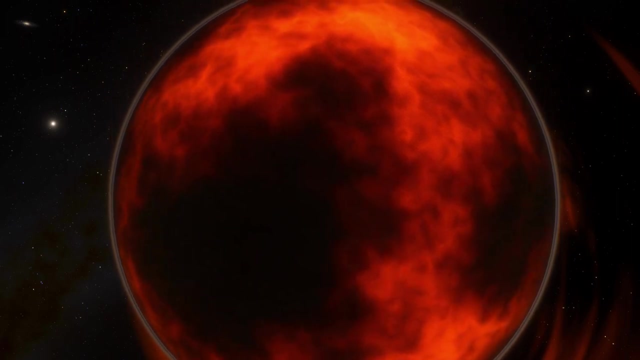 few hours, Once captured light can be probed to determine the composition of exoplanet atmospheres. Consider a prism: When you shine white light through it, it splits the light into a rainbow spectrum. The color bands of the spectrum can be: 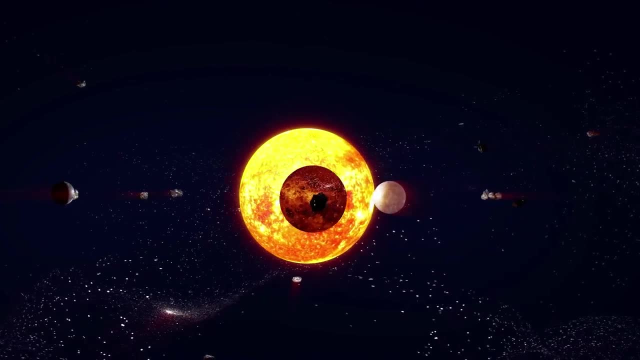 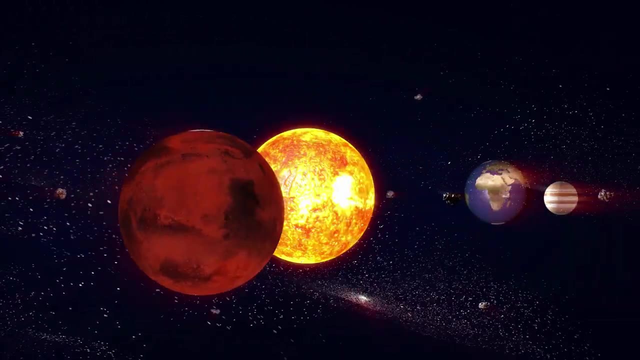 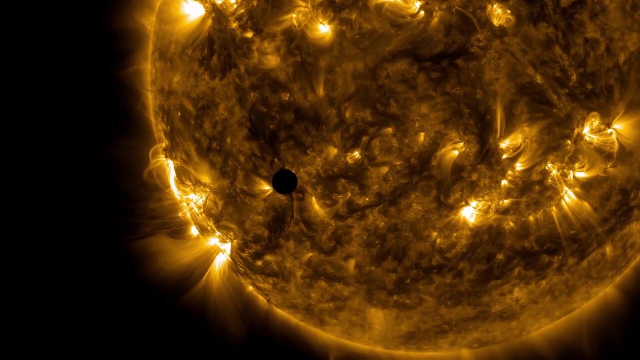 read by scientists like a barcode revealing which molecules are present. It's a technique known as transit spectroscopy, in which light from a star travels through the atmosphere of an orbiting planet and reaches our telescopes in space or on the ground, telling us where it's been. The transit 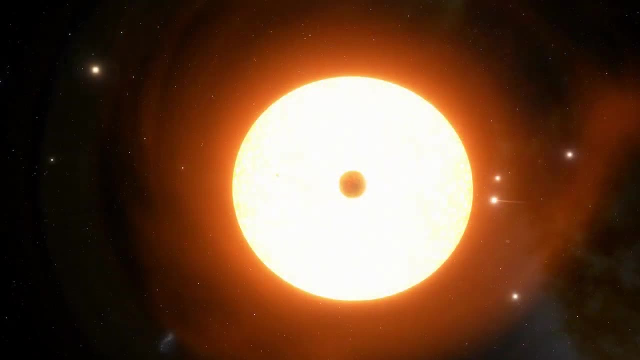 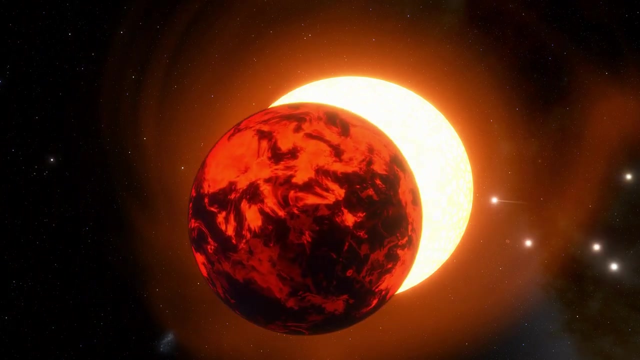 timing variation method takes into account whether transits occur with strict periodicity or whether there is variation. When multiple transiting planets are detected, the transit timing variation method is frequently used to confirm them. Transit duration variation refers to changes in the duration of the 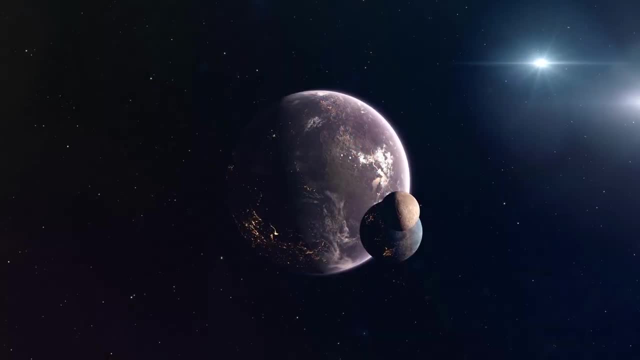 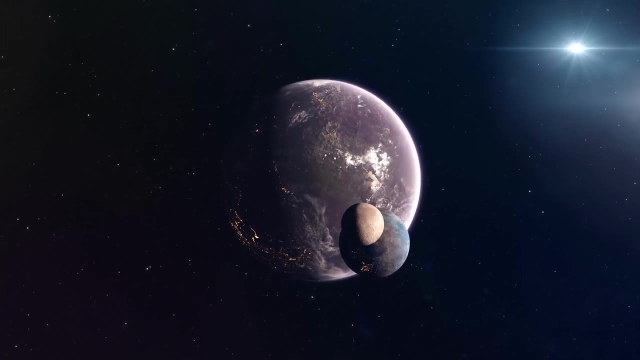 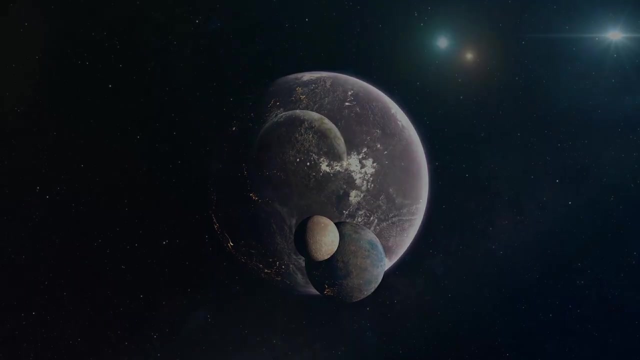 transit Exomoons, absolute precession for eccentric planets caused by another planet in the same system or general relativity can all cause duration variations. This method is used to detect planetary systems with binary stars. It is a particularly useful method for space-based 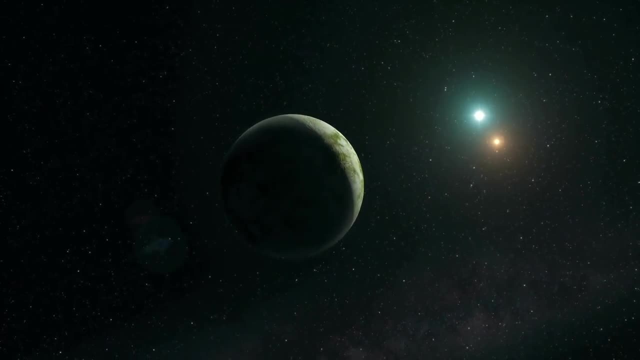 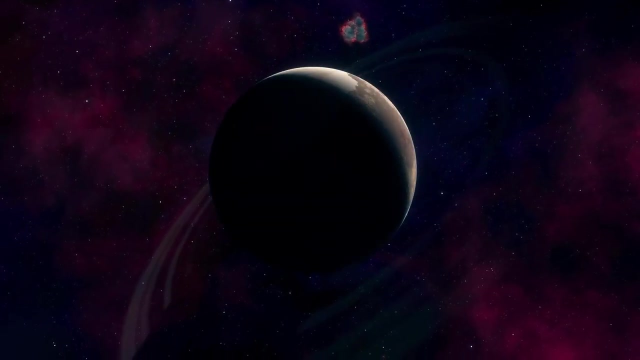 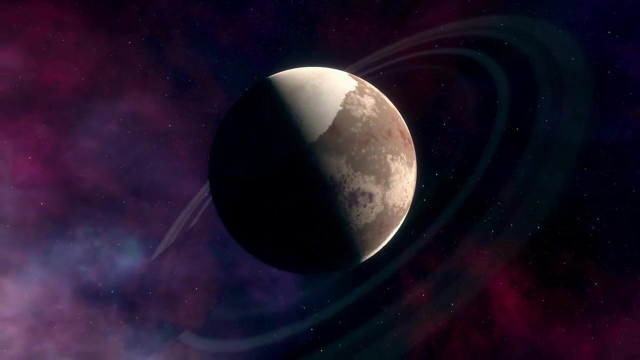 observations. Transits can also detect planetary systems that can stare at stars for weeks or months at a time, although it can be useful for ground-based telescopes as well, This method is good at determining diameter, but bad at determining mass of the planets. 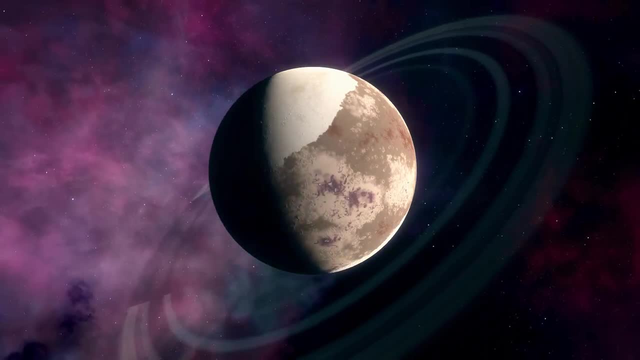 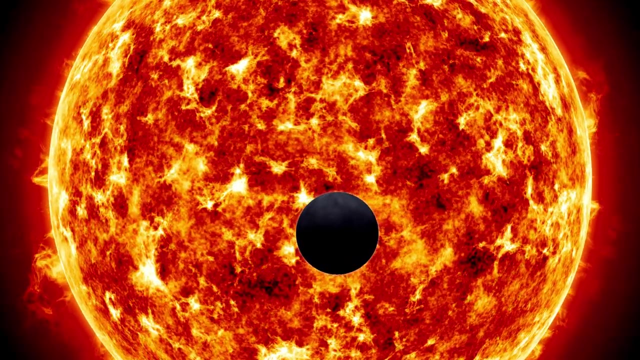 Transit photometry searches can operate on a massive scale. Transit surveys, both ground-based and space-based, can observe up to 100,000 stars at once. The main issue is that the stars are not always as large as the planets in the sky, so they 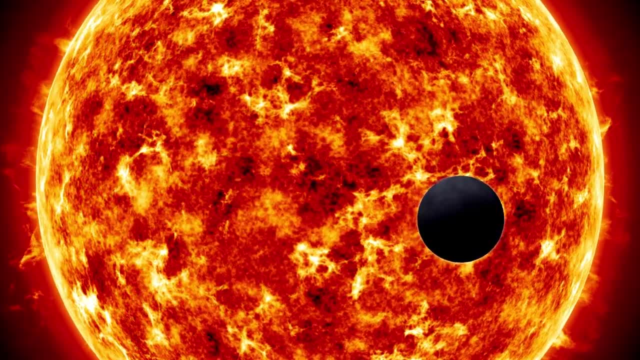 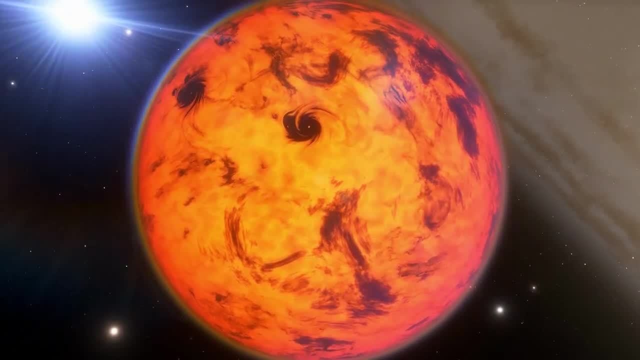 are not always as large as the planets in the sky. The main issue with the transit photometry method is that a transit must occur in order for the photometric effect to be measured. A distant planet must pass directly between its star and Earth. Not all planets orbiting other stars transit their stars. as seen from Earth. Another issue is that a planet's transit only lasts a fraction of its entire orbital period. A planet's orbit may take months or years to complete, but the transit is likely to last only hours or days. As a result, even if astronomers observe a star with a transiting. 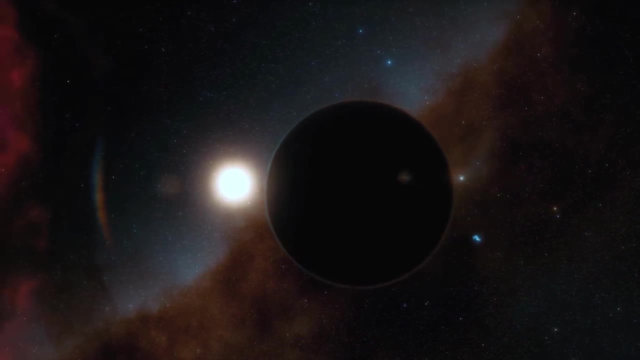 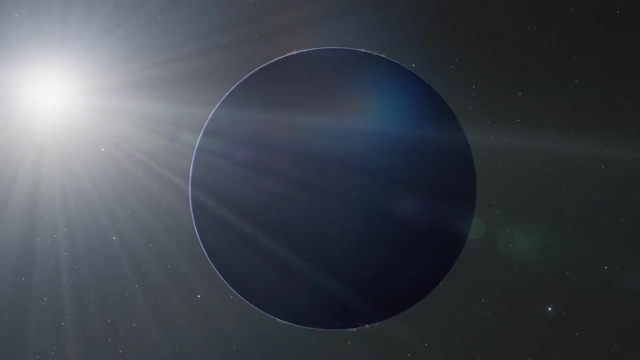 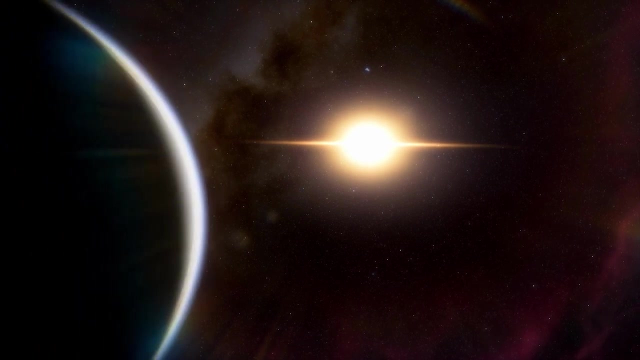 planet. it is extremely unlikely that they with will witness the transit in progress, Because the smallest stars can have diameter similar to giant planets. the transit photometry method frequently produces false positives, Despite its disadvantages. this method is used to find more than 3,900 planets to date. The planet can then be erupted on Earth by 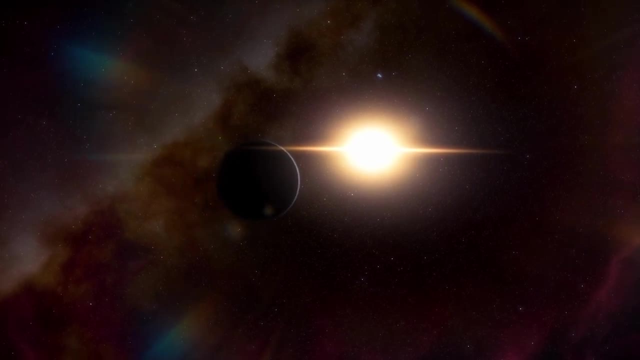 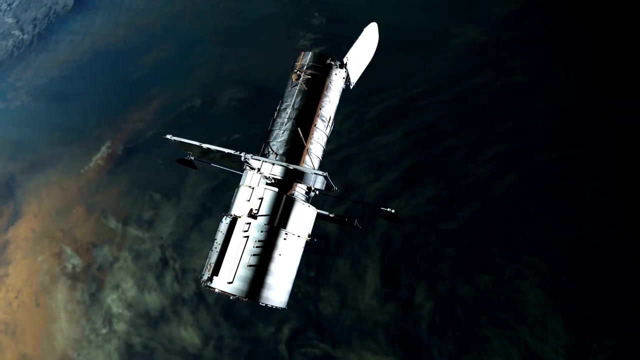 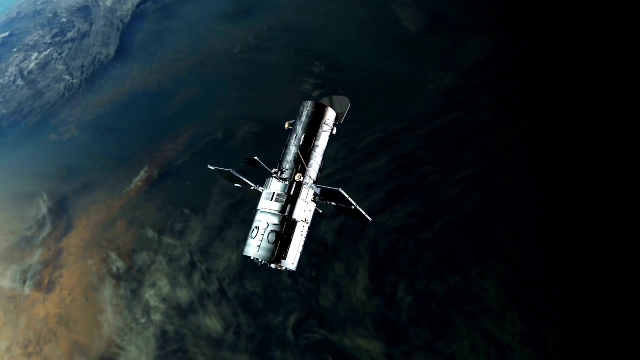 to date and it will help to detect many more in the future. Instruments of Detection. The Kepler Space Telescope heralded the modern era of planet hunting. Kepler entered an Earth-trailing orbit and focused its attention on a small patch of sky. It had been staring at that patch for four years.